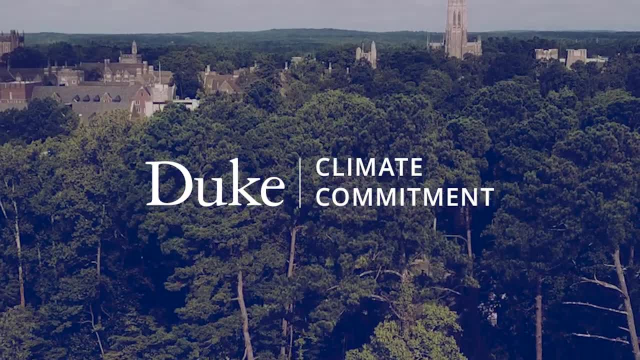 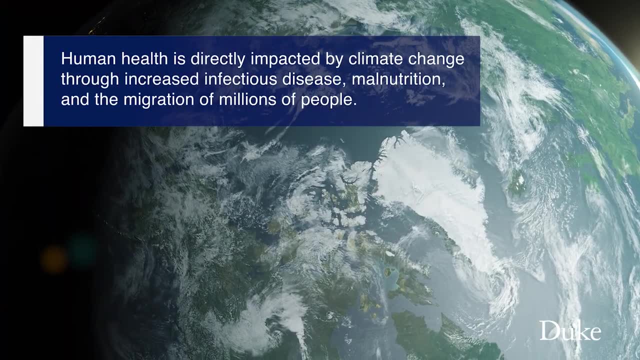 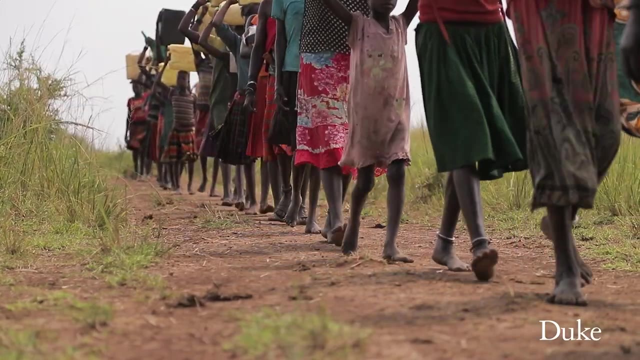 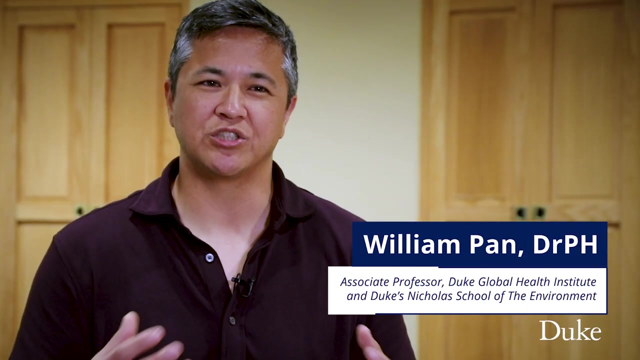 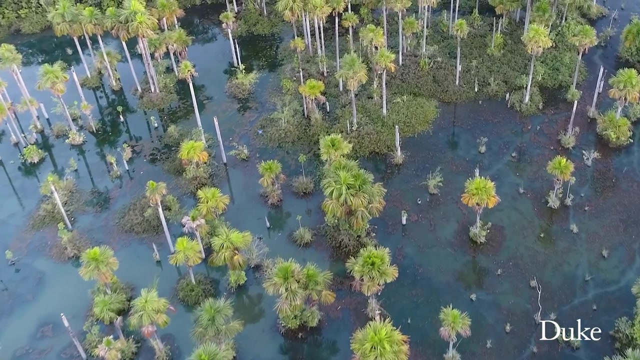 I study malaria primarily in the Amazon, And what happens with climate change. you get changing temperatures on the ground. you get changing patterns of rainfall. That affects where mosquitoes can grow. It affects when mosquitoes can grow and how long their lives last. Climate change influences transmission on a local scale, but also large, regional. 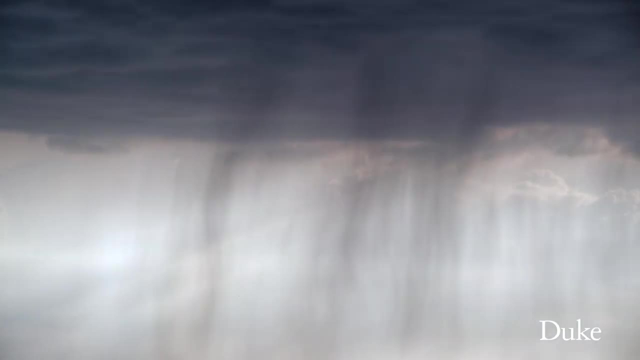 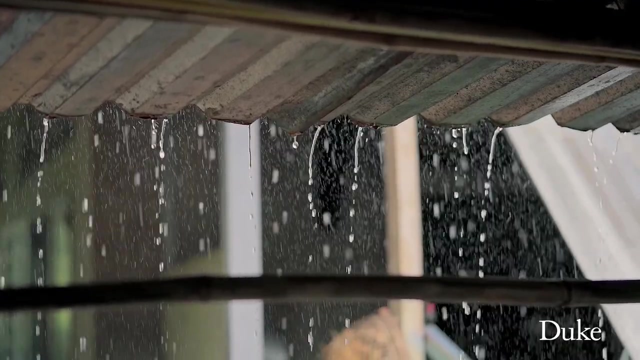 scales. If you move the season earlier and you expand the season, you get more cases of malaria And that's primarily caused by an earlier wet season, which means you have an earlier time of when transmission occurs. The other thing that climate change does with 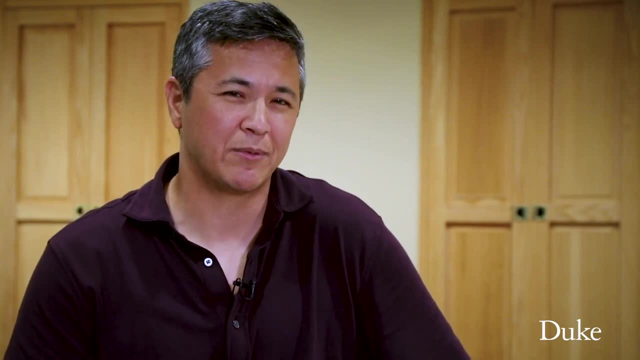 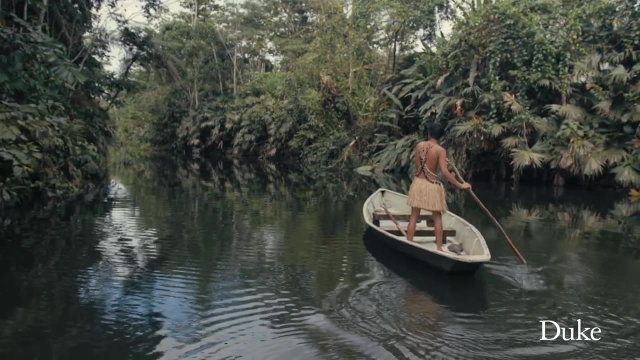 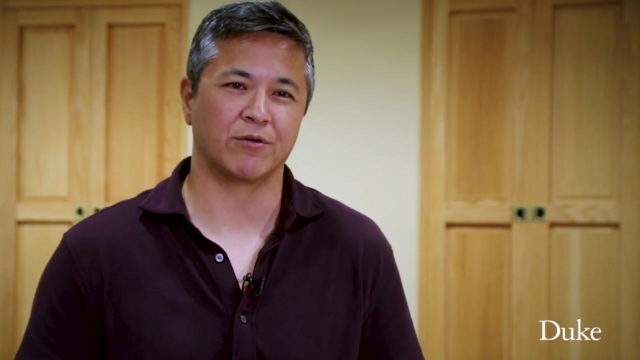 malaria is that it really influences how people move across a landscape, especially in the Amazon, since migration and mobility is highly tied to river heights, So that can control how much migration occurs on a landscape, which is directly related to how much malaria you view and observe in one particular area versus another. 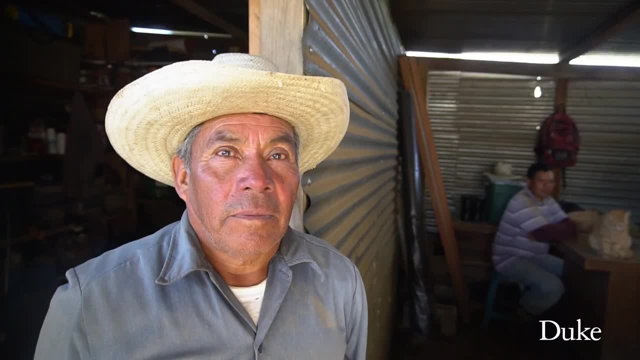 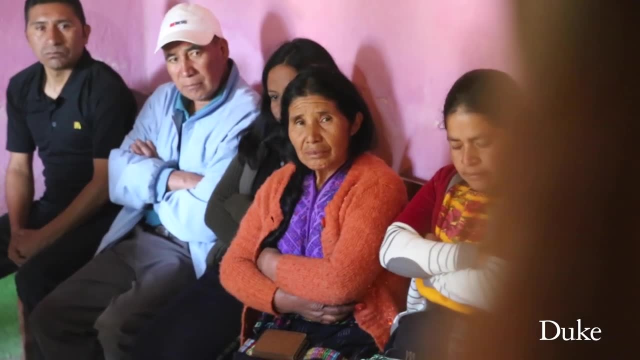 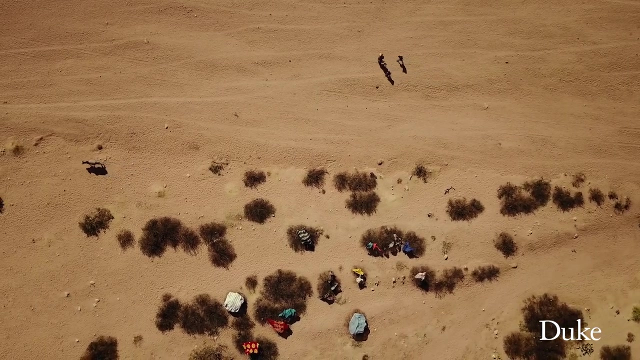 Climate migrants. they're escaping an area not because of a political or a violent threat, but because they can't create a livelihood to survive, And so they're making these choices to hike through really harsh conditions to get out and try to make a better life. We. 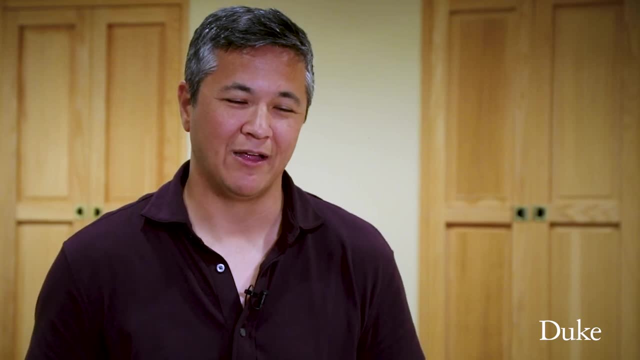 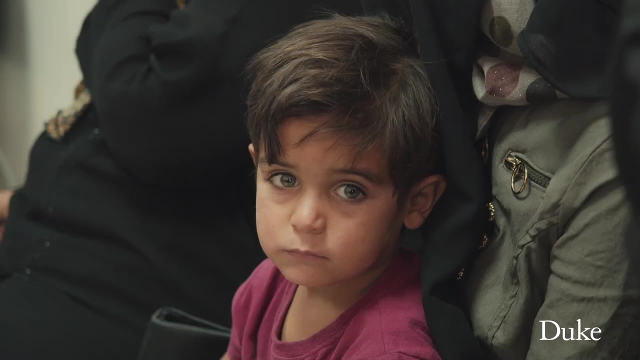 need to better understand why climate migration is occurring And, from a health perspective, we need to do a better job of providing health care to refugees, to help them get out of refugee camps, to make sure that they're receiving the care that they need: One Health. 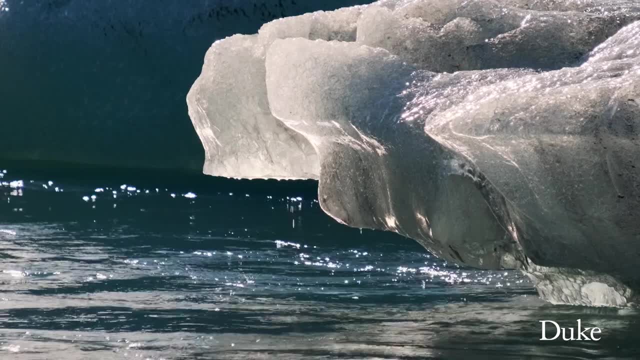 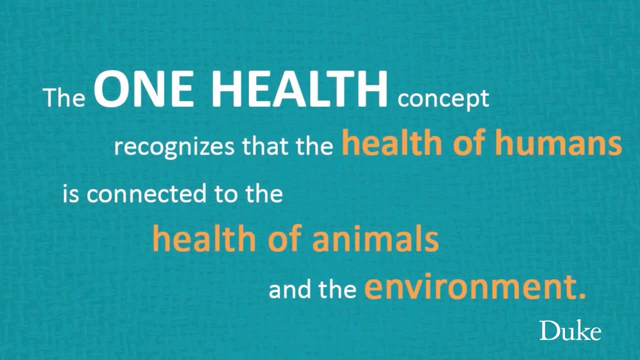 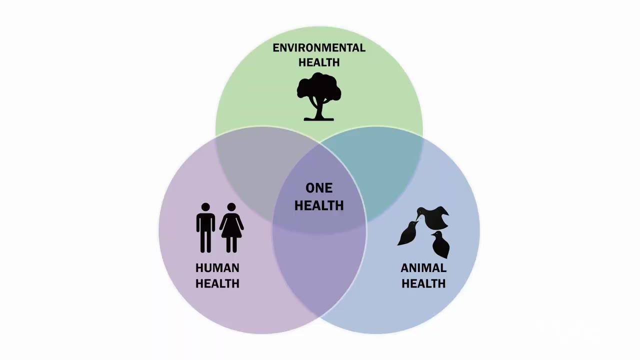 is a really important way of viewing how we, as humans, are tied together with the environment. So things that happen in any one of those realms, any of the human-animal-environment realm, impacts the other two and is applied to things like infectious disease. It's applied.